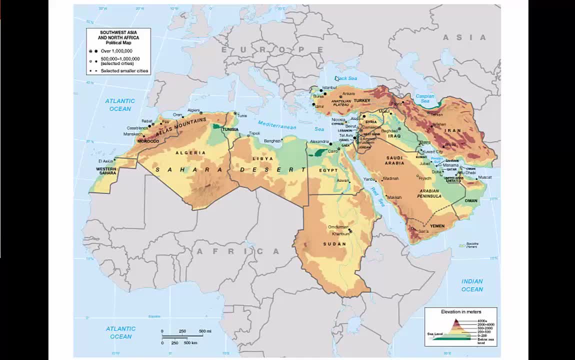 with Southwest Asia, or sometimes the term Middle East. that extends from Iran all the way over to Western Sahara. These are more religious connotations here. The major religion here is going to be Islam. We can look at some of these regions here where the actual 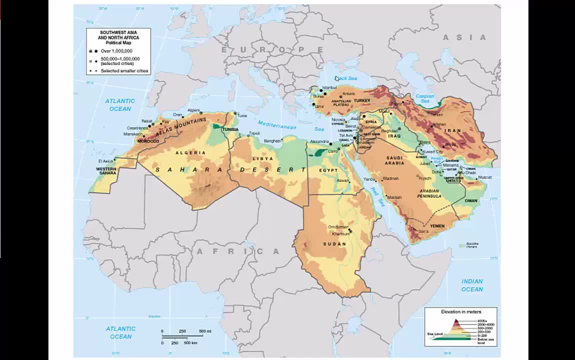 continents are divided up and we'll see these with Central Asia, South Asia, Southeast Asia. This is a particular area we're looking at here. Sudan- here I alluded to before. we've got a South Sudan right here. that was created in 2011.. My previous map did have that This. 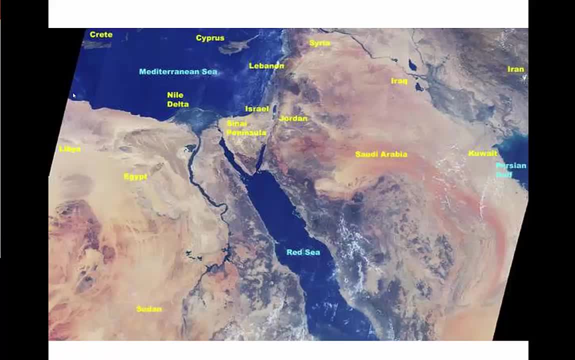 is what we look at here. This is a satellite image that we're looking at of the large area here extending from Libya over to Kuwait. You can see these green areas are obviously going to be vegetated. 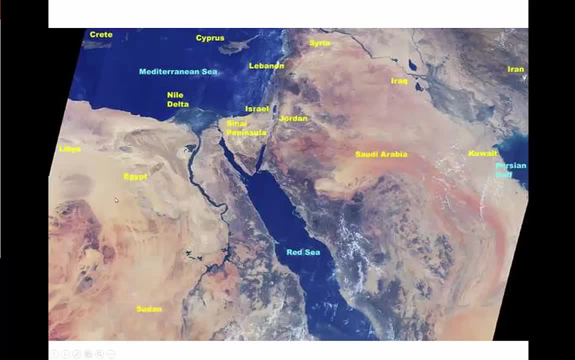 but a lot of desert. You can see the Sahara Desert right here that serves as that large barrier between Sub-Saharan Africa and Northern Africa. It is the underlying physical barrier that we deal with. desert, rather, is in this whole region. here We'll talk about the politics. 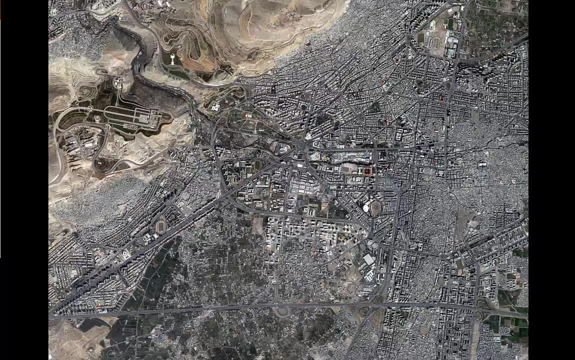 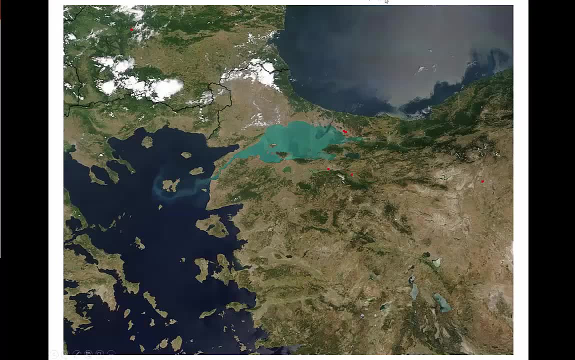 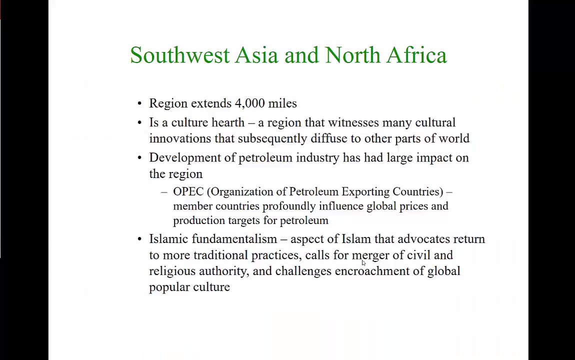 of water in part of this. 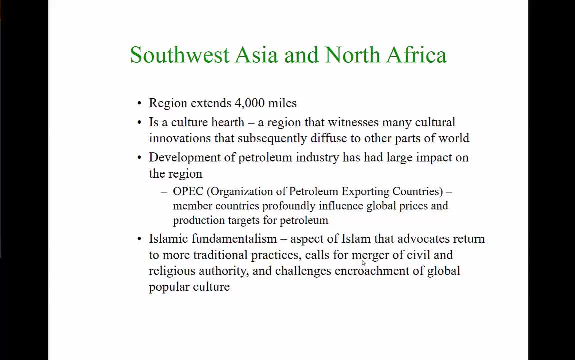 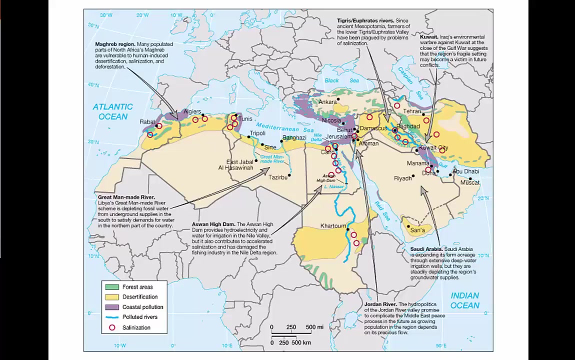 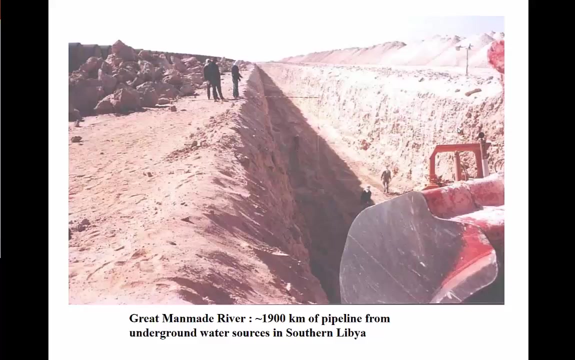 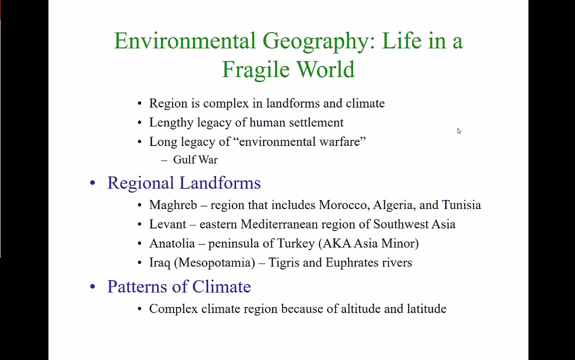 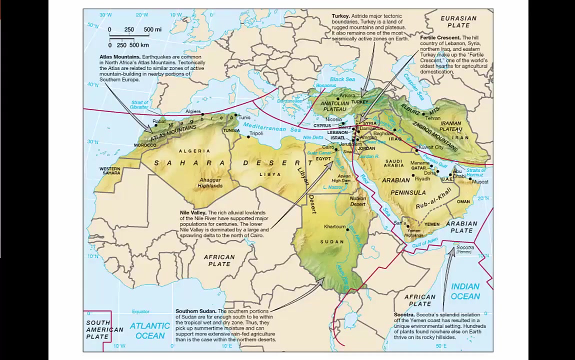 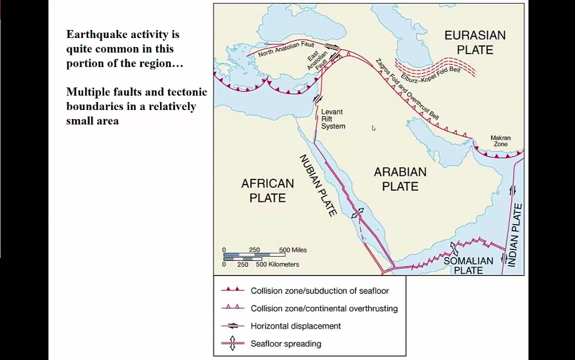 There's a lot of earthquake activity. In the last decade we've had earthquakes in Iran. 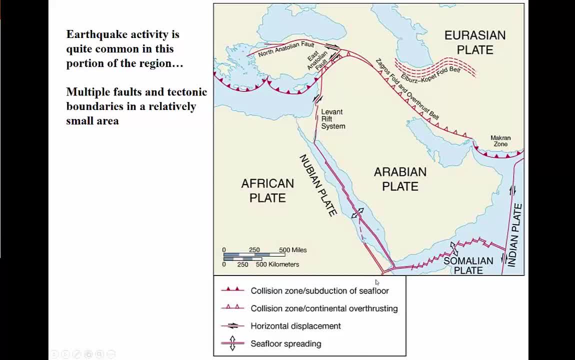 But like we have this divergent zone here in Eastern Africa, that African Rift Valley, we've got a spreading center right in the middle of the Red Sea here And then we have a convergent plate boundary right in the middle of the Mediterranean Sea. 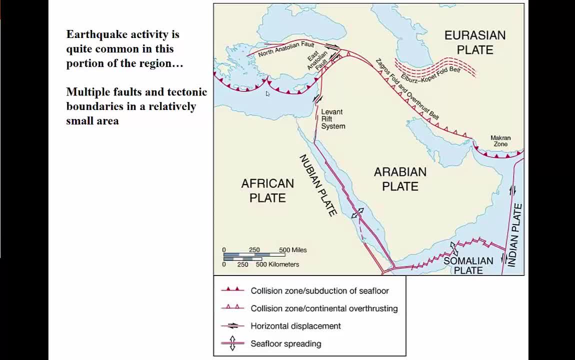 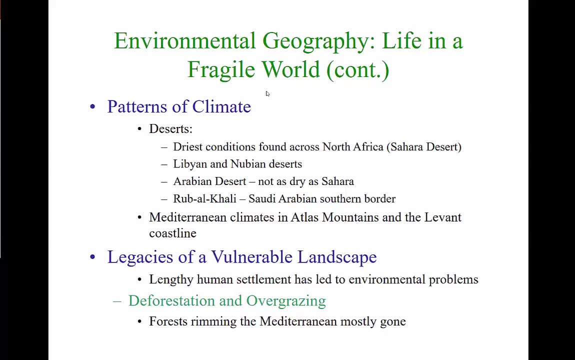 So places like Iran, even Saudi Arabia, Saudi Arabia and Turkey are major locations for tectonic activity. Underlying theme is deserts, especially in northern Africa: Sahara Desert, Arabian Desert, not quite as dry. Then you've got some Mediterranean climates in the Atlas Mountains and the Levant coastline. 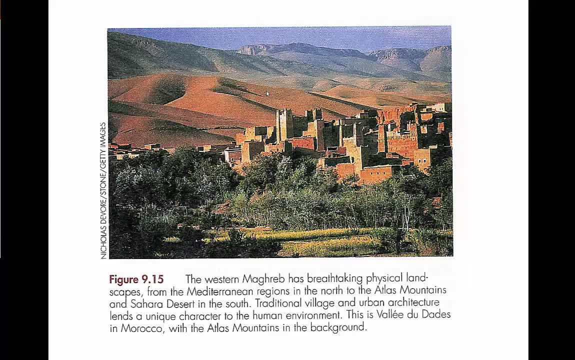 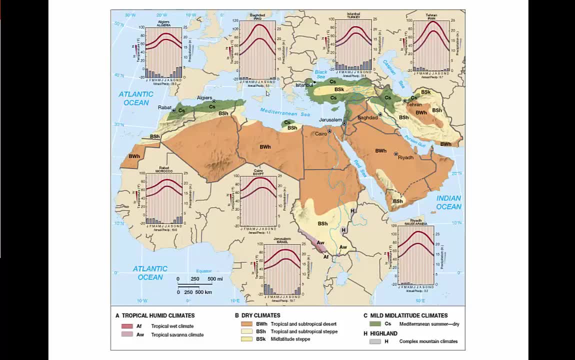 And you can see some of the regions that we're looking at here. This is in Morocco, And then you can see the climate. A lot of bees, which represent our desert, are dry, But we do have a couple of these seeds here. the Mediterranean and summer dry. 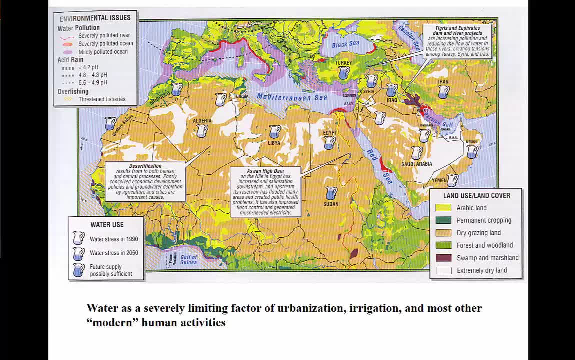 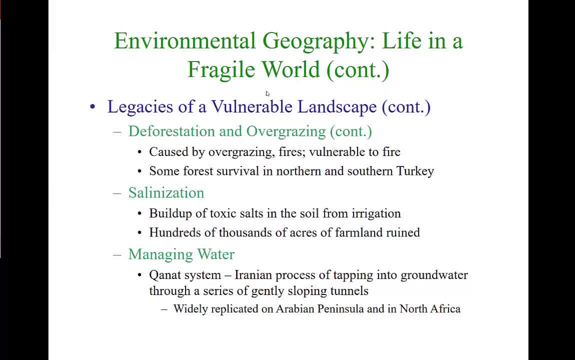 Like I said before, water is a limiting factor of urbanization, irrigation and most other modern human activities getting water to these particular places. That's very important. And then these are just some of the issues with environmental geography These days: mankind's impact on the environment. 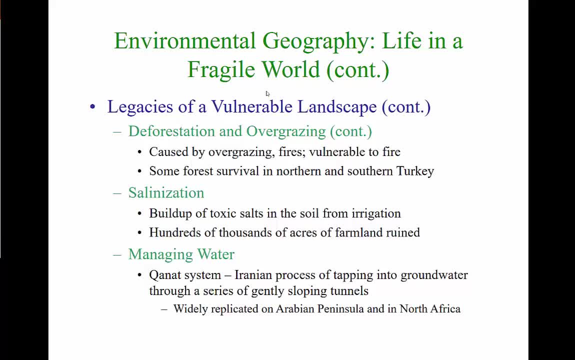 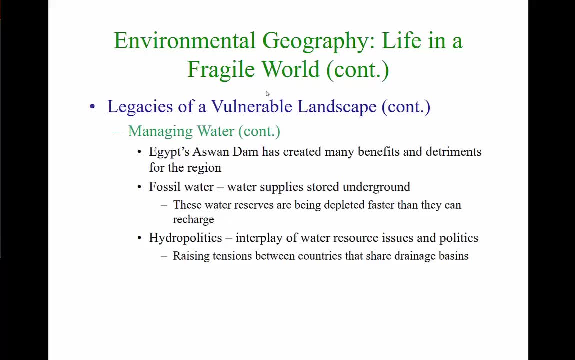 So, combined with how we manage this, as well as the physical geography that we're talking about, We've had the damming of waters, the Hai'aswan Dam, which dammed up the Nile, And then, like I said before, hydropolitics. 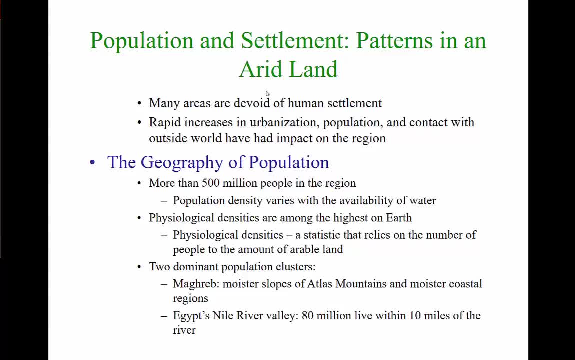 Population: more than half a billion people live in this region, And then the about 80 million people live within 10 miles of the Nile River in Egypt, But a lot of places that are sparsely populated due to this lack of water. 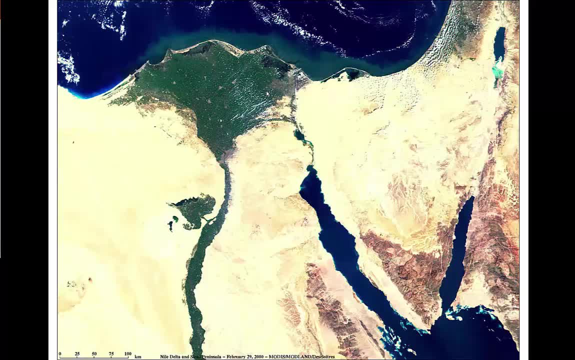 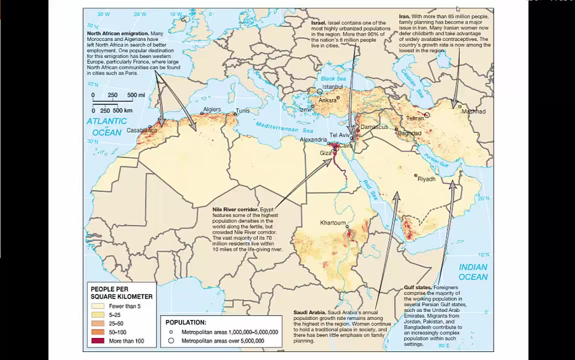 Thought this was interesting. This is from a MODIS imagery, But you can look at Egypt here in the Sinai Peninsula, Right here as we move over here to Israel, And then, looking at a dot density map, we can see where people are located. 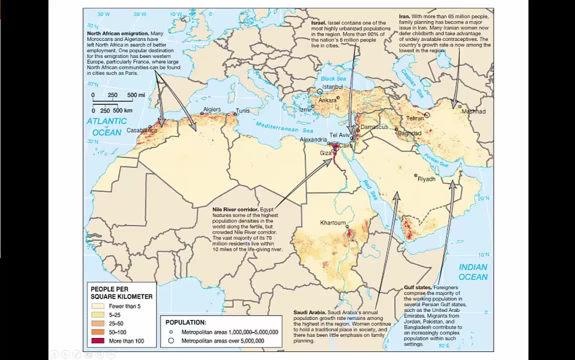 So along the coasts, here you can see the Nile River Delta, right here You can see the Middle East. here We've got Syria, Egypt, Iran, And then, right tucked in, here is Israel, And then, Moving south, we've got Sudan. 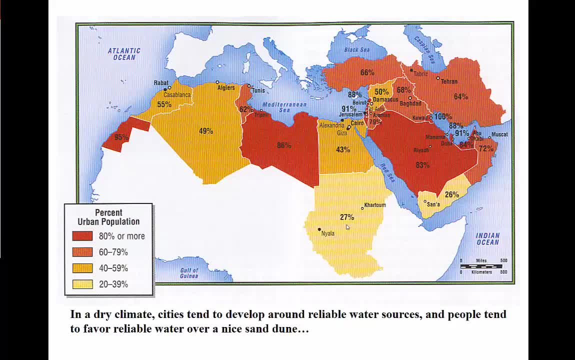 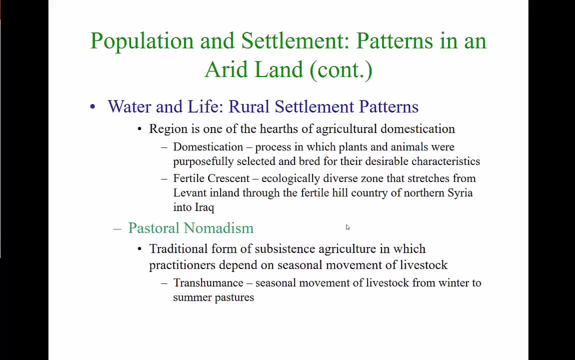 Then we can look at the percent urban as a result of this, And a lot of this is based on this access to water. So this slide gets into some of the rural sediment patterns as a result of water, The whole idea of pastoral nomadicism. 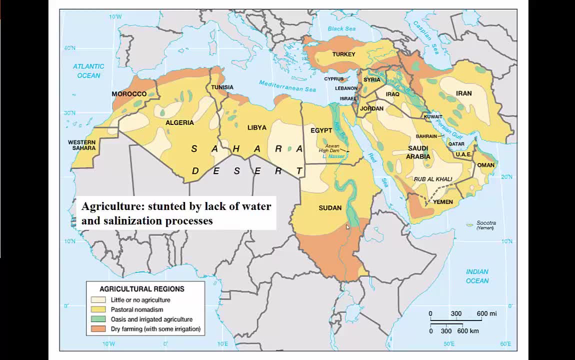 You know, in these days, you know there's a lot of lack of large scale desalinization plants. I know this region is one of the areas trying to get into the whole idea of eliminating salt from water, but it's still costly and resource intensive. 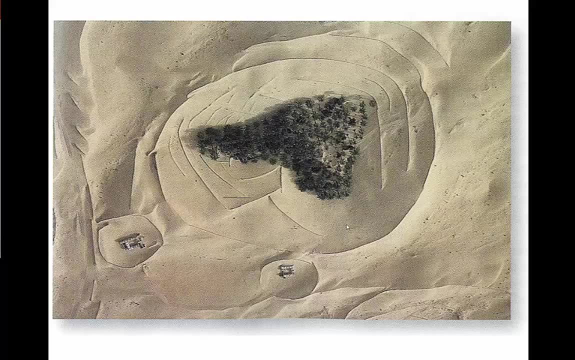 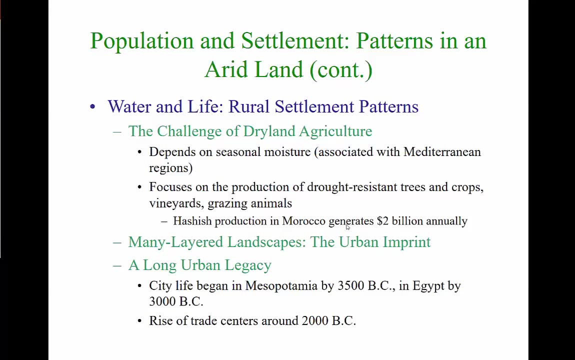 Oases, So you can see some of these oases where there is water. And then this talks about the challenge of dry land agriculture and the whole idea of you know urban centers, How you know Urban regions and urban legacies. 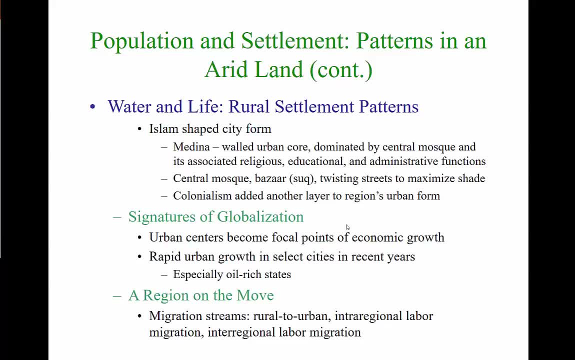 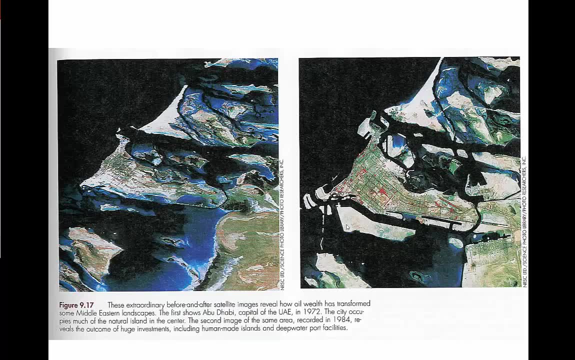 Be it again. Thought this was neat. These are some satellite images of Dubai. Oil has transformed this region economically, So this is an Abu Dhabi, the capital of United Arab Emirates. So you can see the the manipulation of the land, And I've got some imagery here. 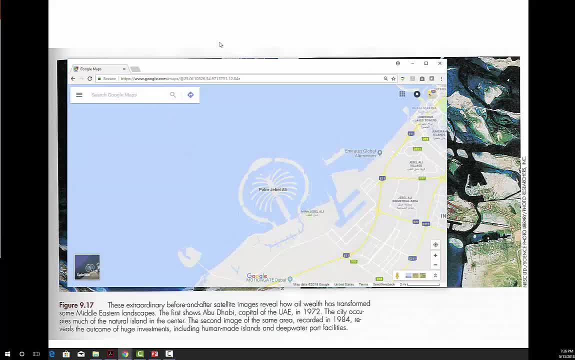 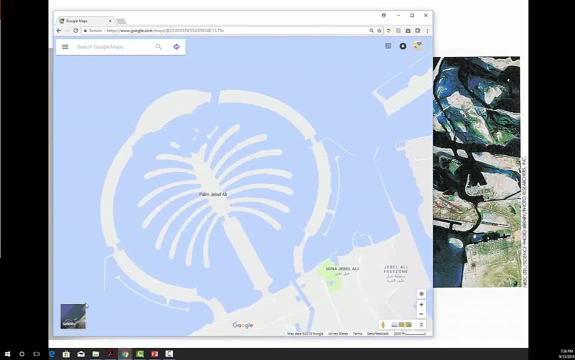 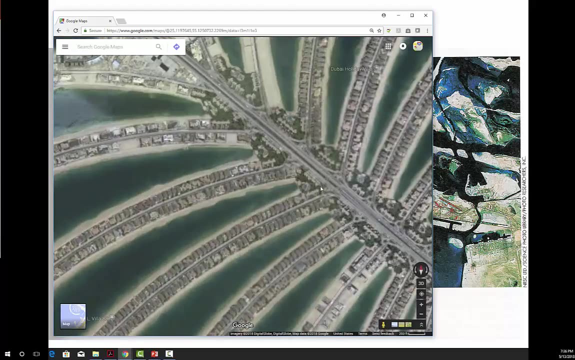 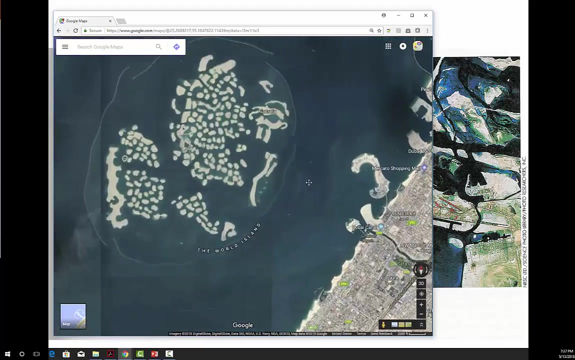 which i thought was neat from google maps. this is in the city of dubai and you can look at these amazing islands here- man-made islands, you know, just absolutely amazing. you know they're taking the sand from out here and creating these lands. here's another one here. these are actually individual islands that. 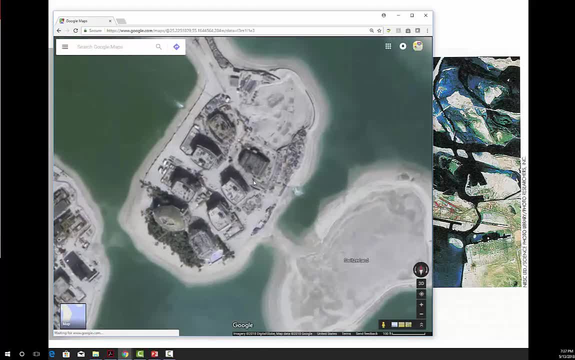 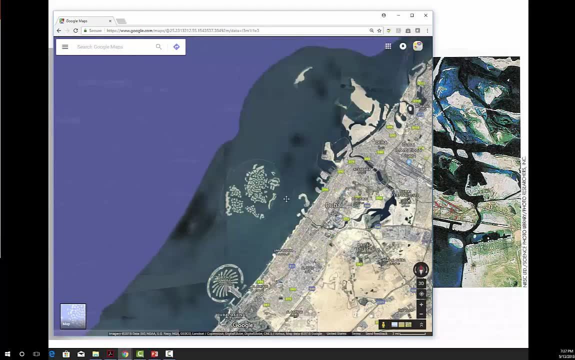 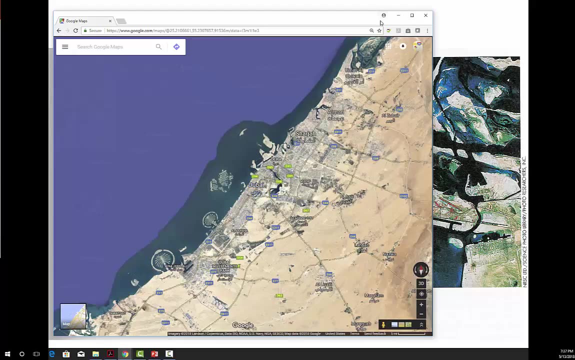 people can live on. i thought these were amazing, and a lot of this proliferation is due to the oil industry. so these are one of the areas that are central to oil, the manufacturing of oil and our dependency on oil, and especially the middle east. so these are some of the places there. 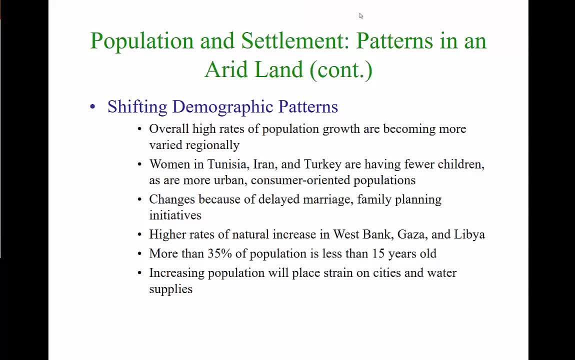 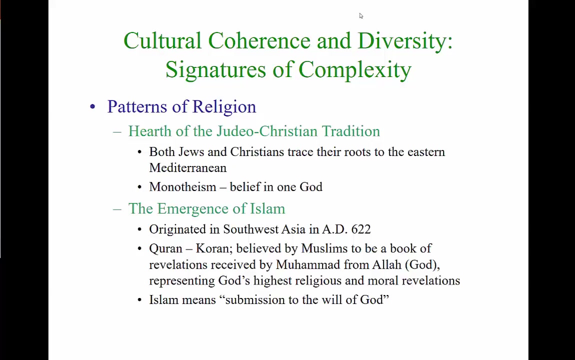 skyscrapers, skyscrapers. and then we have shifting demographic patterns. okay, it's not quite as stark as africa, but we still have a fairly young population. so this increasing population is going to place a strain on cities and water supplies. it's the hearth of judeo-christian, uh, judeo-christian tradition. 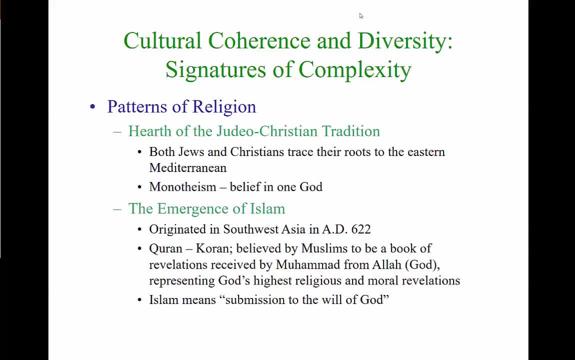 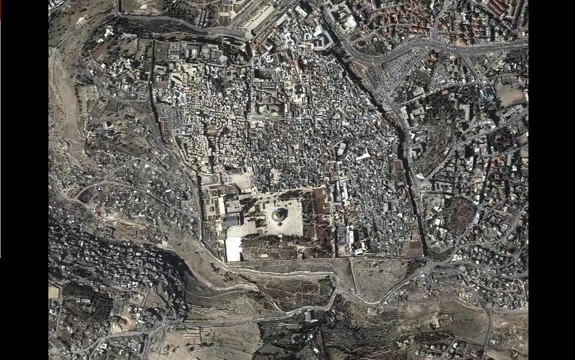 as well as the emergence of islam. so this is, you know, the center for a lot of your major. you know what we- i think the term is abrahamic religions, and you can see jerusalem here and you can see the modern religions. so we have islam. 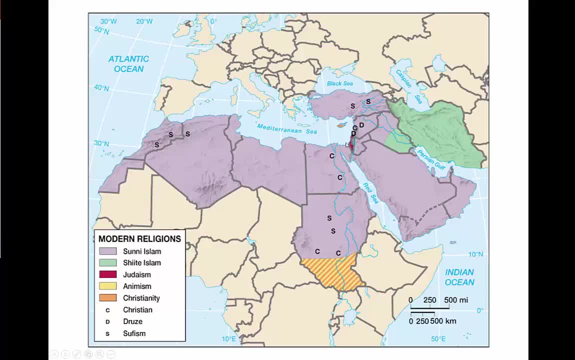 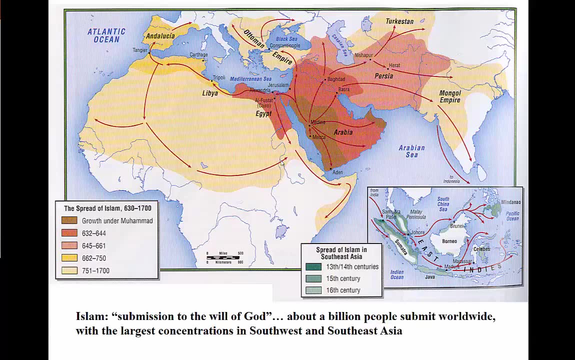 the two different sects of islam. we've got judaism here and we do have some christianity around some other regions here. then we can see the spread of islam over time. okay, and like i think i alluded to before, indonesia is actually the most populous. 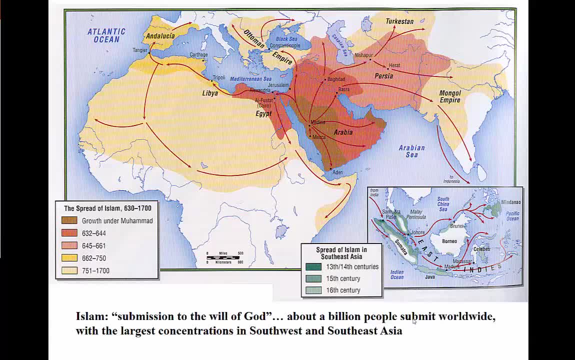 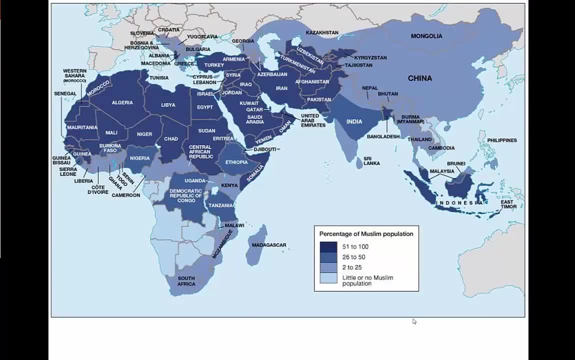 muslim nation. they're not percentage-wise but the actual number of people, since indonesia is the fourth most populated country in the world and just looking at this percent islam, so we can see this whole idea of distance decay. you know, further away you get, the less from the hearth you can see some of the issues. 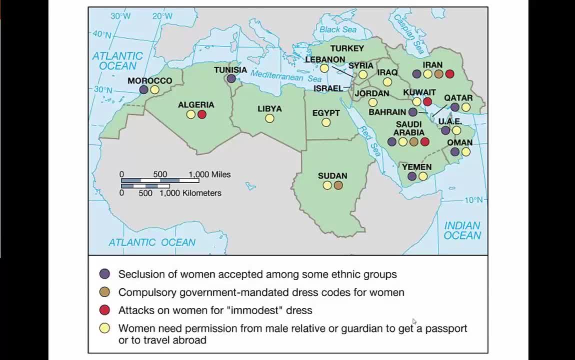 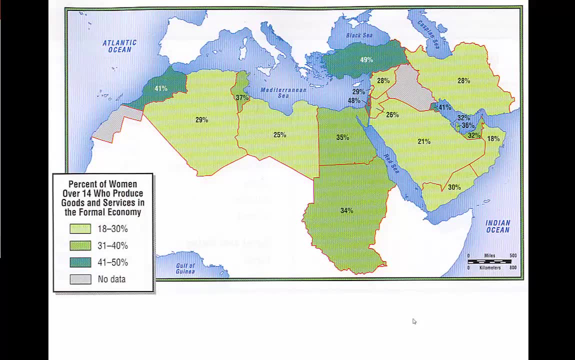 related to the status of women in some of these countries. and then economy: we can see some of the economic, and you know, the participation of women in goods and services in our formal economy in these particular countries. religious geography: you know, like i said before, there's a lot of theocracies. 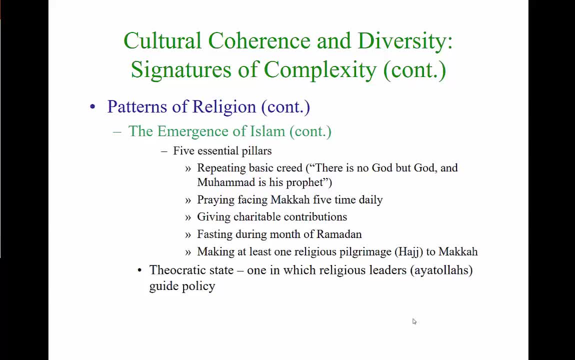 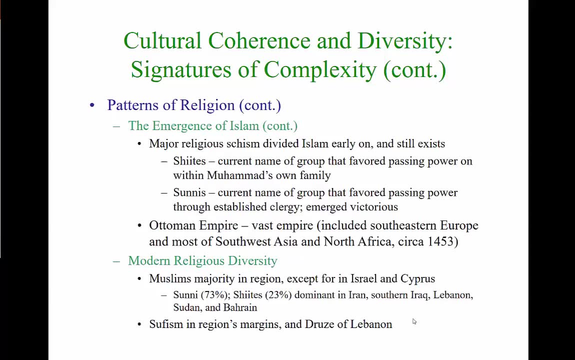 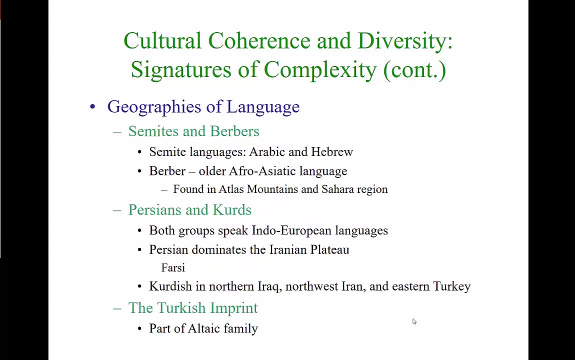 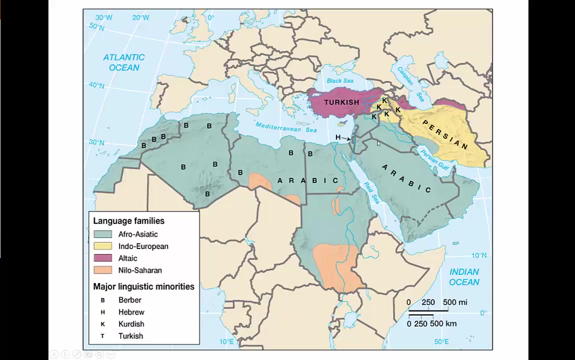 meaning. you know, these are religious leaders who also run these countries, so this talks about these: the differences between religions and women right, different divisions, other types of culture, groups, and then the language families here. And then we can see Kurdish- and we've heard that term, Kurdistan from Iraq, but this is 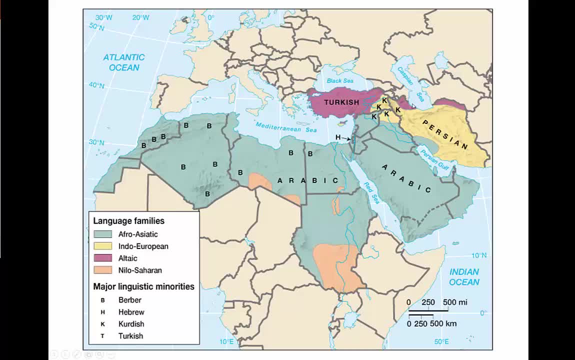 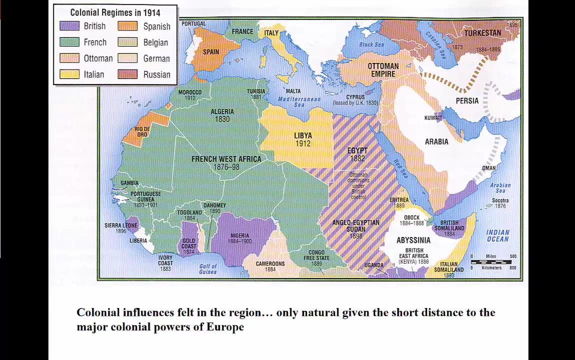 a nation here, but it's a minority in Iran, Syria, Iraq and Turkey, so they don't make up a majority in any one of these countries. And then the colonial influences here. So over here in the Middle East we can see the Ottoman influence. we've got French over. 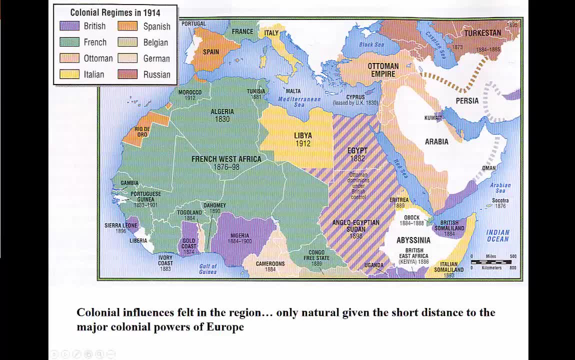 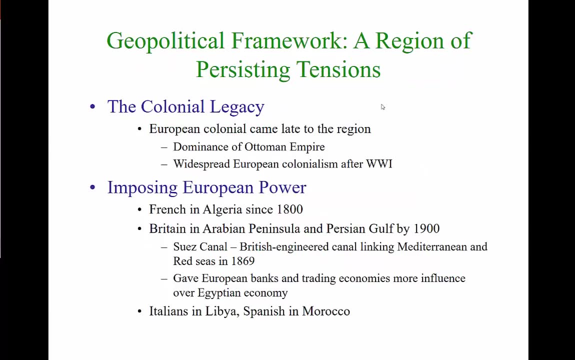 here we've got Spanish, Italian here with Lydia, and then the British influence here with Egypt. Like I mentioned before, Before the colonial influence, the Suez Canal that was manufactured by the British or engineered by the British to link the Mediterranean and the Red Sea, so people didn't have to. 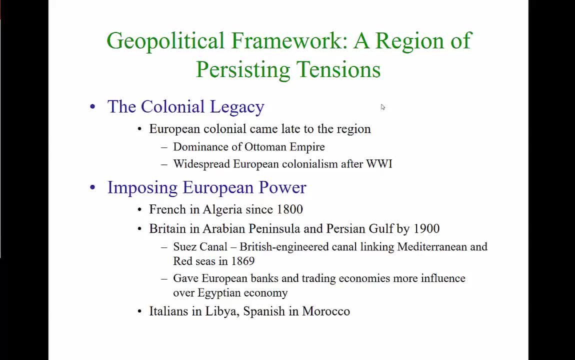 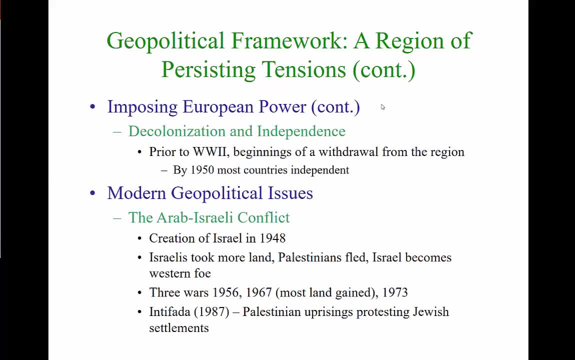 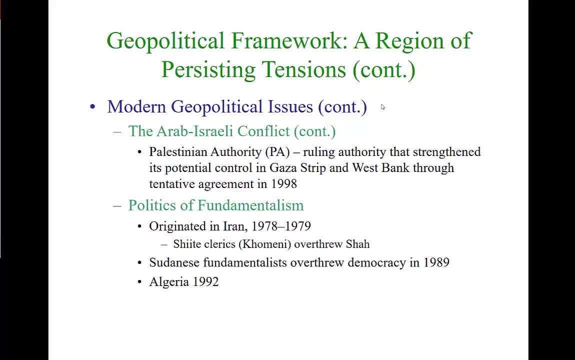 go around Africa, But there's Italians in Libya, the Spanish in Morocco, And then, these days, some modern geopolitical issues: Creation of Israel in 1948.. Politics of fundamentalism: This is something that we hear about A lot these days. 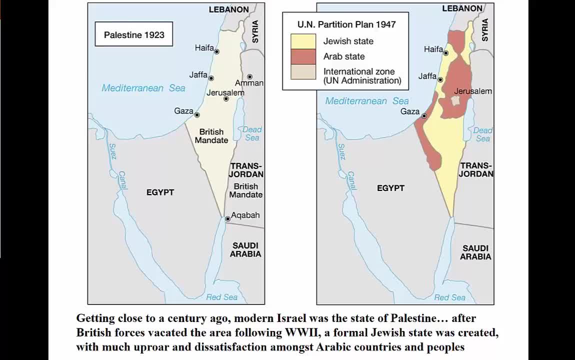 And then you can see the growth of Palestine, which turned into the Jewish state in 1947, and who knows where we are with that now in 2018.. We do have Gaza Strip, we have West Bank, we have Golan Heights, and they do have some. 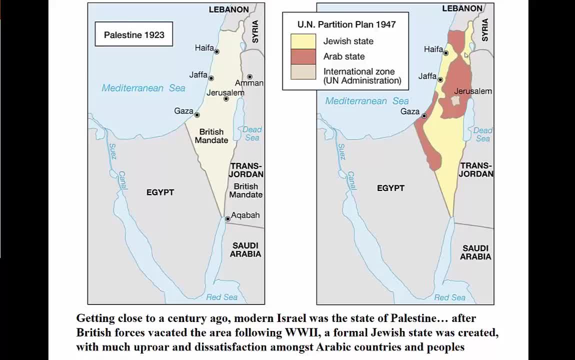 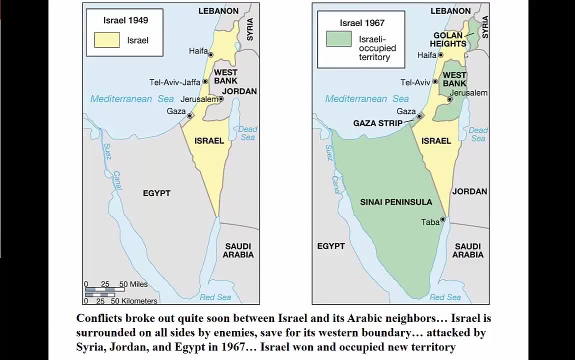 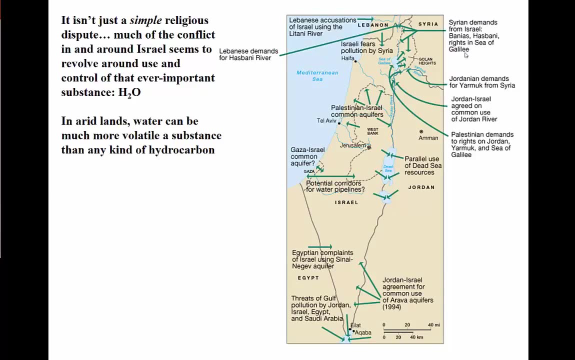 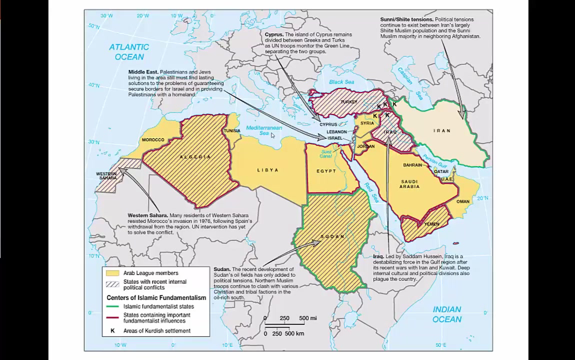 level of autonomy, but they're not formally recognized as individual countries as yet, And then you can see how this has gone on throughout the years. So you can see some of the hydro politics of this particular region here, And then some of the countries with internal conflicts. 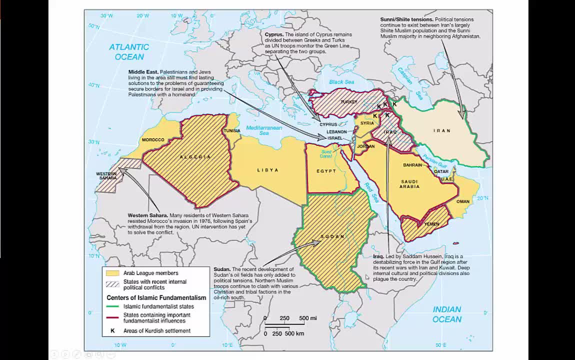 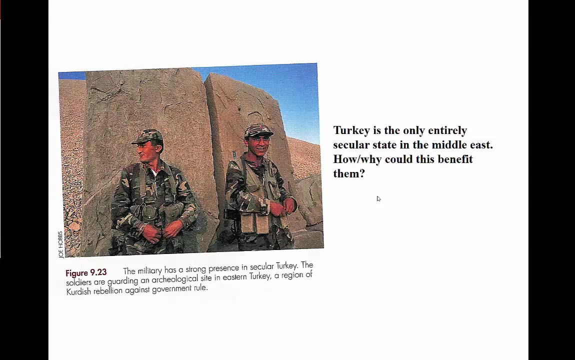 You can see this alludes to Sudan. There is now a new country called South Sudan, One of the least developed countries in the world right now looking to get a foothold. And then Turkey's, the only entirely secular state in the Middle East, meaning it's not. 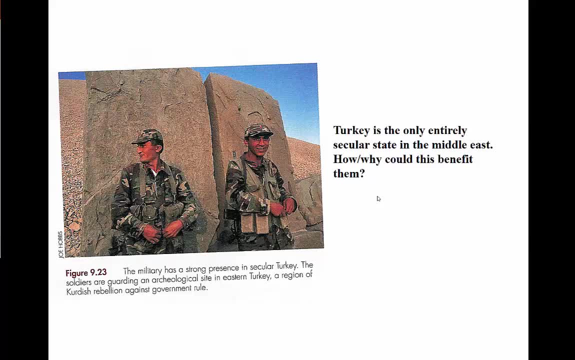 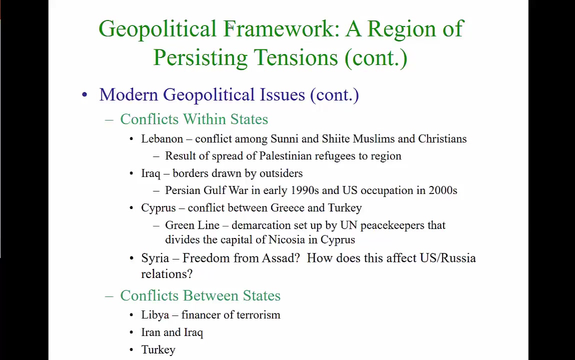 theocratic Religion has little play in the actual running of the government, even though it's largely Islam. And then you hear about Turkey days, especially with Syria, since Syria is very nearby other things- the Cyprus. it's split between Greece and Turkey. there's something called the green line. 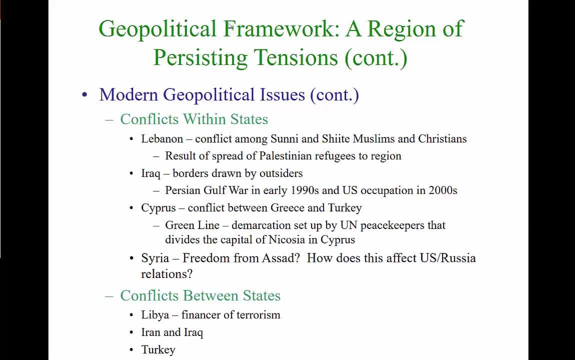 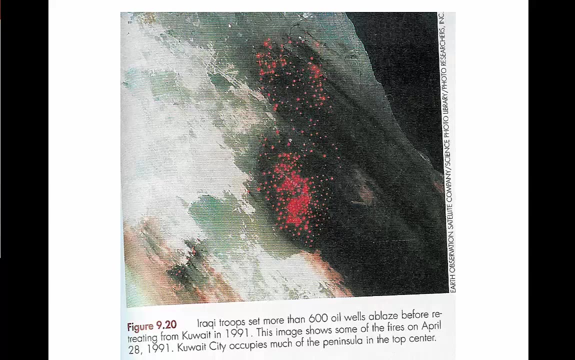 Syria. we hear about that in the news- freedom from Assad. how does this affect the US and Russia relations? some of the geopolitics we saw before in the 90s we had the Gulf War, so Iraqi troops when they retreated from Kuwait because they invaded Kuwait. this shows some of the imagery and the environmental. 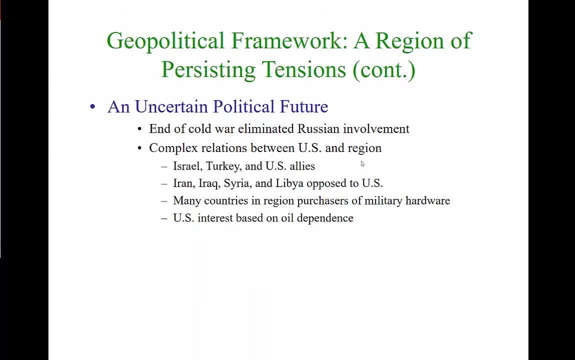 degradation as a result of that and then just some uncertain political futures. you know Iran and Iraq. you know Iran and Iraq. we're in a war throughout the 80s, you know, and how does this affect us? you know how does affect relations and a lot of the US interest based on oil. 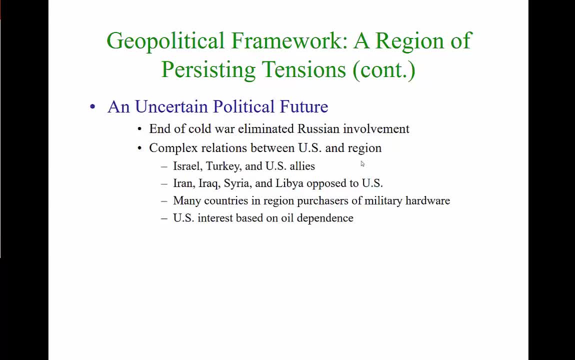 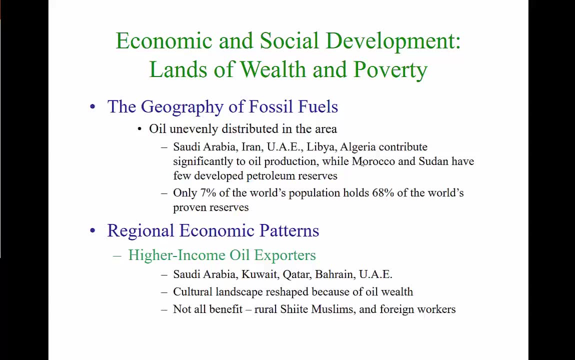 dependence. so it'll be interesting and to see how this moves in the future and, like I mentioned before, the geography of fossil fuels and then what's going to happen when we start to migrate to renewable energy sources, what's going to happen to these countries and we're going to start to see more of oil being a part of- and you know that's. 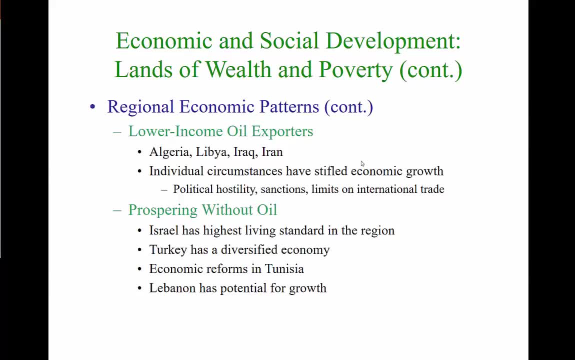 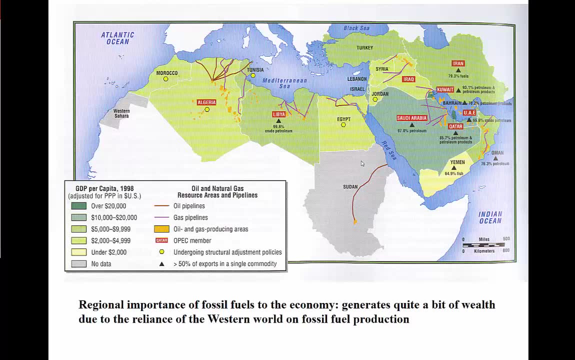 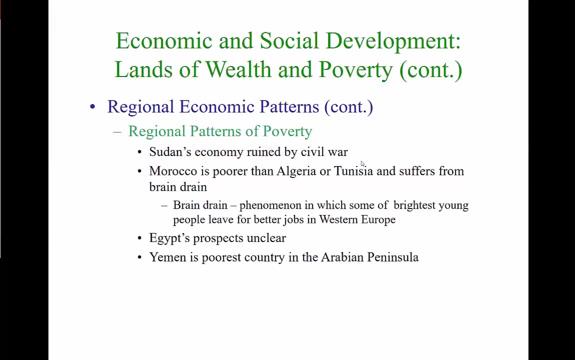 something we're really keen to see and I think it's going to be really interesting and in a lot of ways, it's going to be very important in the future as well. so you can see the crude petroleum reserves, natural gas preserves, just the importance of fossil fuels, yeah, as a wealth generator, and then you know it.